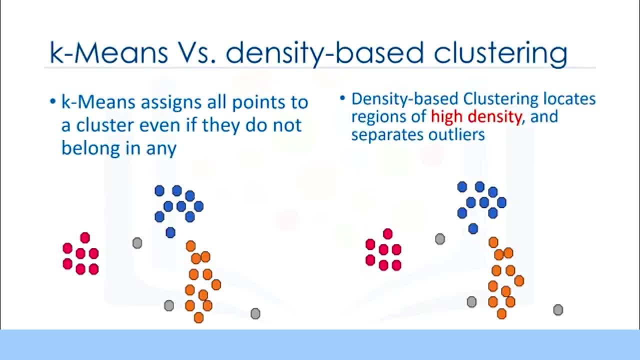 or the performance may be poor. Additionally, while partitioning-based algorithms such as k-means may be easy to understand and implement, in practice, the algorithm has no notion of outliers, That is, all points are assigned to a cluster even if they do not belong in any. 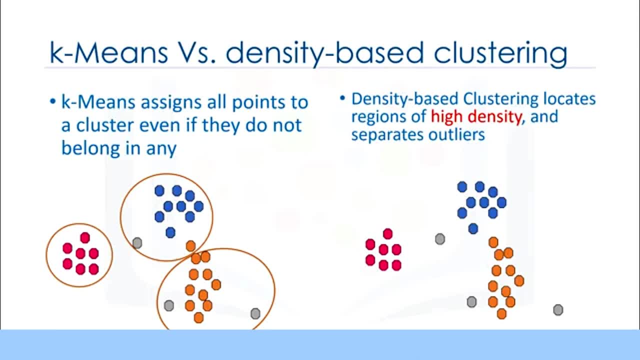 In the domain of anomaly detection. this causes problems, as anomalous points will be assigned to the same cluster as normal data points. The anomalous points are assigned to the same cluster as normal data points. The anomalous points are assigned to the same cluster as normal data points. 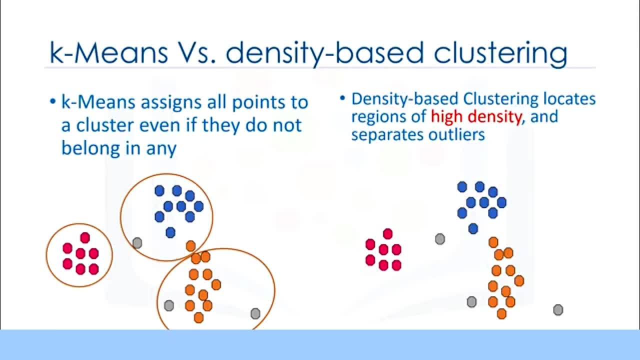 points pull the cluster centroid towards them, making it harder to classify them as anomalous points. In contrast, density-based clustering locates regions of high density that are separated from one another by regions of low density. Density in this context is defined as the number of points within a specified. 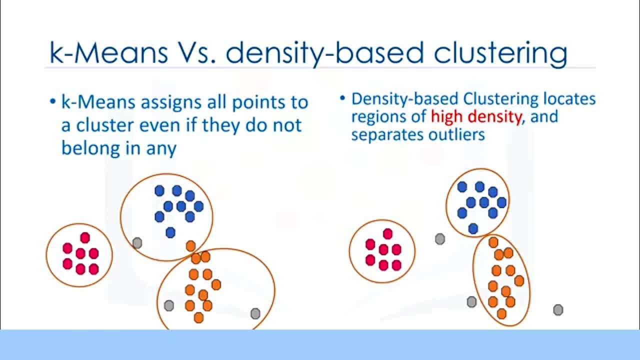 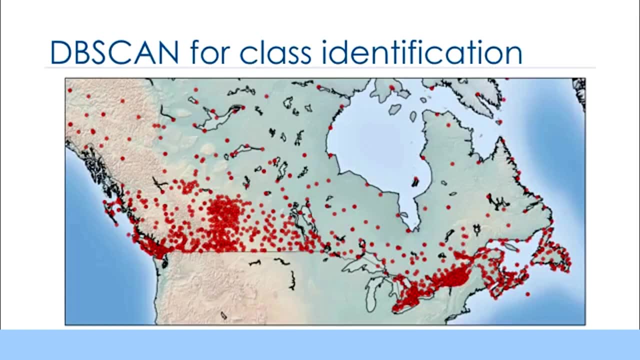 radius. A specific and very popular type of density-based clustering is db-scan. db-scan is particularly effective for tasks like class identification on a spatial context. The wonderful attribute of the db-scan algorithm is that it can find out any arbitrary shaped cluster without getting affected by noise. For 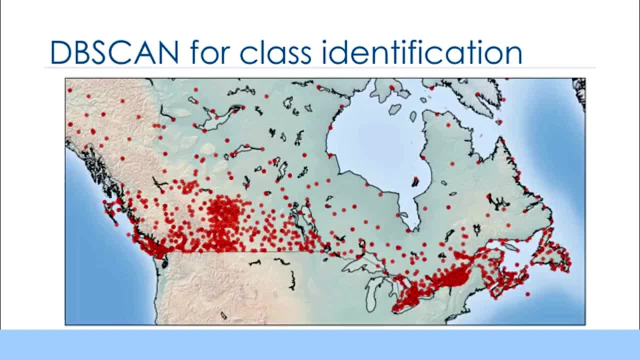 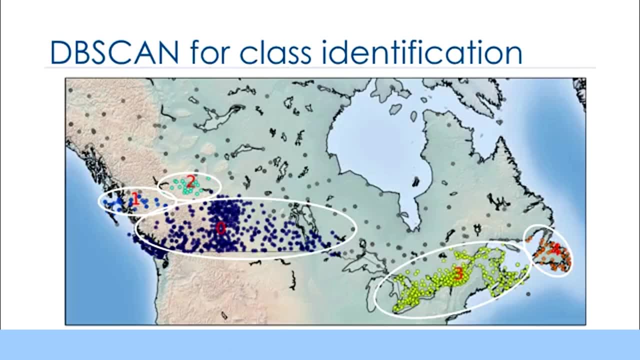 example, this map shows the location of weather stations in Canada. db-scan can be used here to find the group of stations which show the same weather condition. As you can see, it not only finds different, arbitrary shaped clusters, it can find the denser part of data-centered samples by ignoring less. 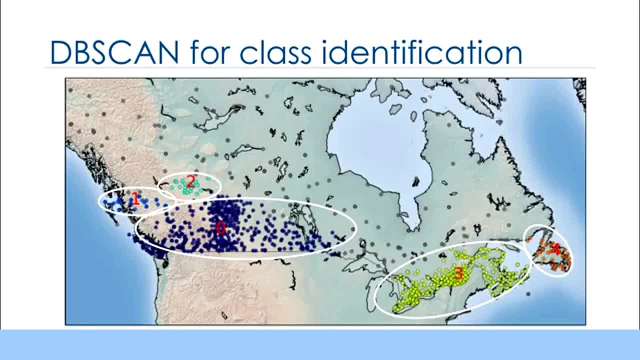 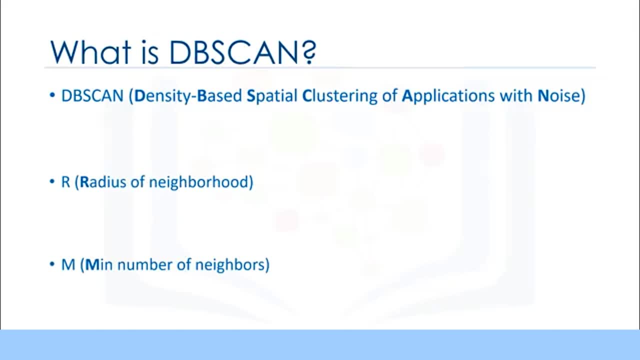 dense areas or noises. Now let's look at this slide- db-scan is a clustering algorithm- to see how it works. db-scan stands for density-based spatial clustering of applications with noise. This technique is one of the most common clustering algorithms, which works based on density. 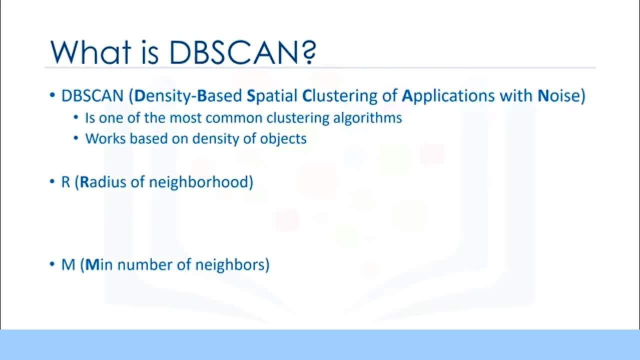 of object. db-scan works on the idea that if a particular point belongs to a cluster, it should be near to lots of other points in that cluster. It works based on two parameters: radius and minimum points. R determines a specified radius that, if it includes enough points. 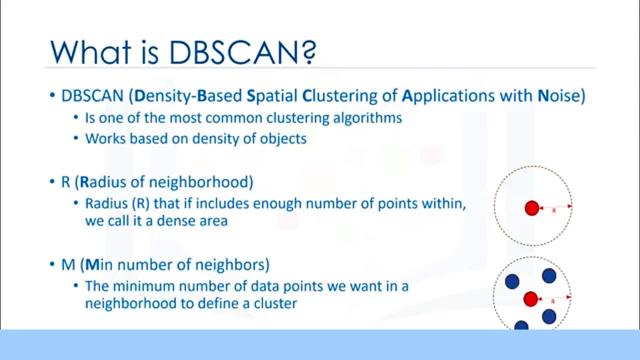 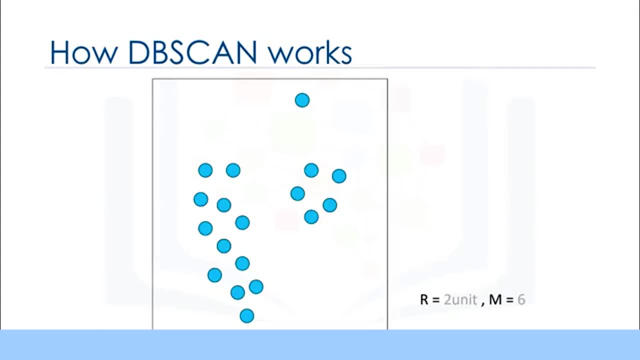 within it. we call it a dense area. M determines the minimum number of data points we want in a neighborhood to define a cluster. Let's define radius as two units For the sake of simplicity. assume it as radius of two centimeters around a point of interest. Also, let's set the minimum point, or M, to be six. 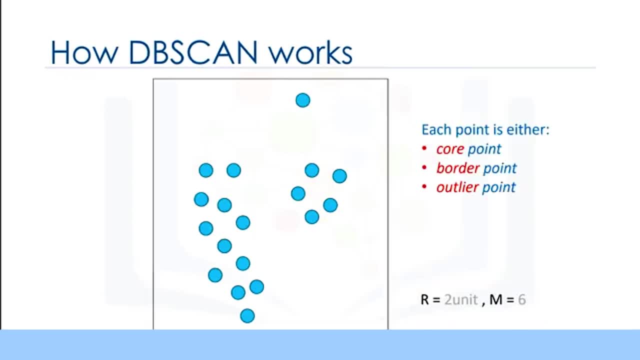 points, including the point of interest. To see how db-scan works, we have to determine the type of points. Each point in our data set can be either a core, border or out-point. For example, we have a group layer point. Don't worry, I'll explain what these points are in a moment. 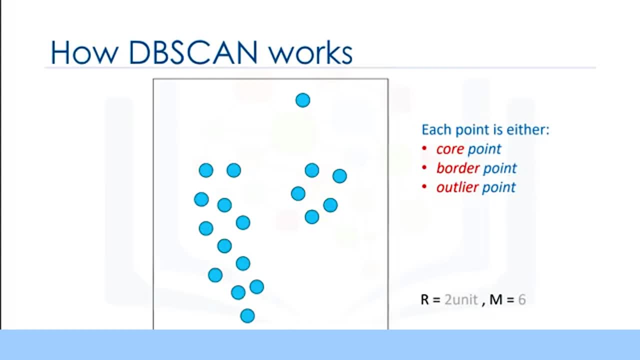 But the whole idea behind the db-scan algorithm is to visit each point and find its type first. Then we group points as clusters based on their types. Let's pick a point randomly. First we check to see whether it's a core data point. So 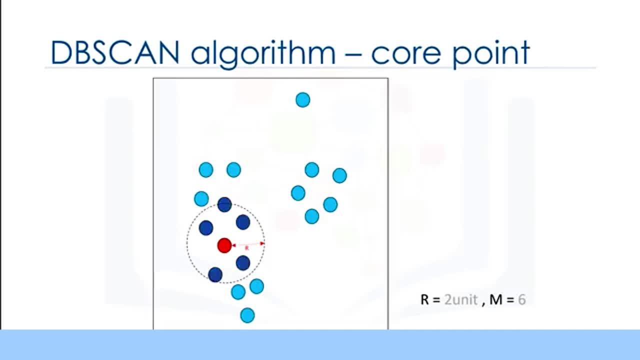 what is a core point? A data point is a core point if, within our neighborhood of the point, there are at least M points. For example, as there are six points in the two centimeter neighbor of the red point, we mark this point as a core point. 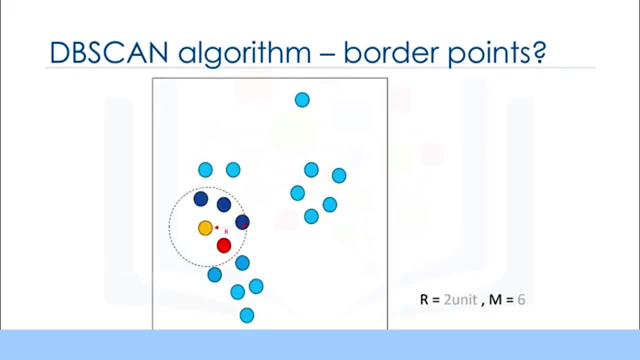 Okay, what happens if it's not a core point? Let's look at another point. Is this point a core point? No, As you can see, there are only five points in this neighborhood, including the yellow point. So what kind of point is this one In? 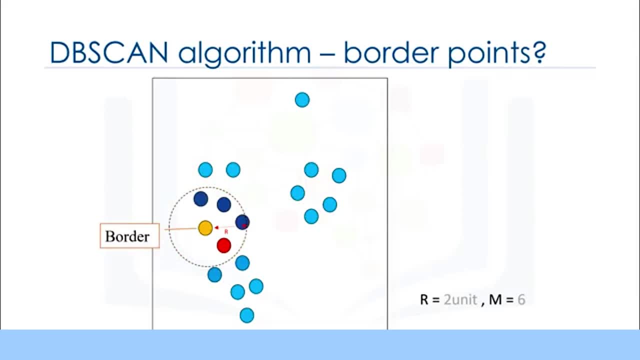 fact, it is a border point. What is a border point? A data point is a border point if a- its neighborhood contains less than M data points or B, it is reachable from some core point. Here, reachability means it is within our distance from a core point. It means that, even though the yellow point is 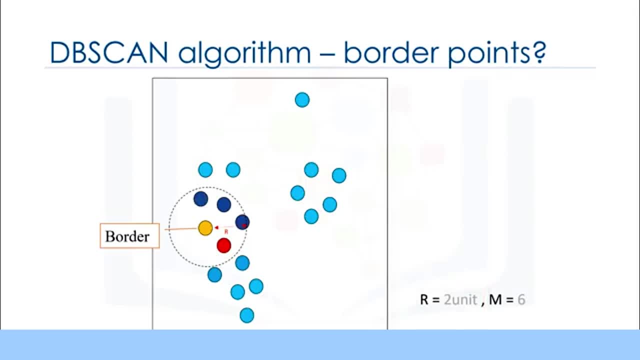 within the two centimeter neighborhood of the red point. it is not by itself a core point because it does not have at least six points in its neighborhood. We continue with the next point. As you can see, it is also a core point And all points. 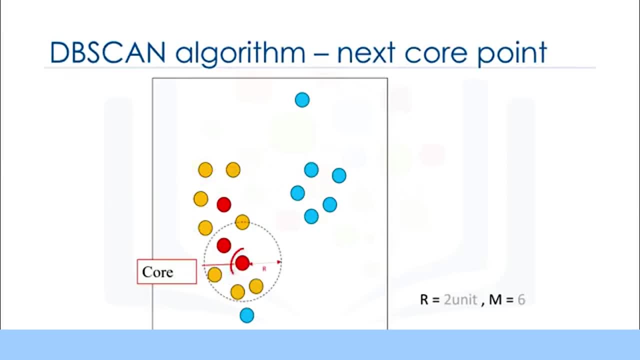 around it, which are not core points, are border points. Next core point And next core point. Let's pick this point. You can see it is not a core point, nor is it a border point, So we label it as an outlier. What is an outlier? An outlier is a point. 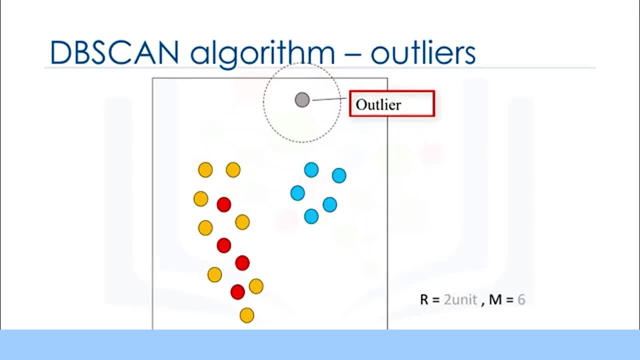 that is not a core point and also is not close enough to be reachable from a core point. We continue and visit all the points in the data set and label them as either core, border or outlier. The next step is to connect core points that are neighbors and put them in.